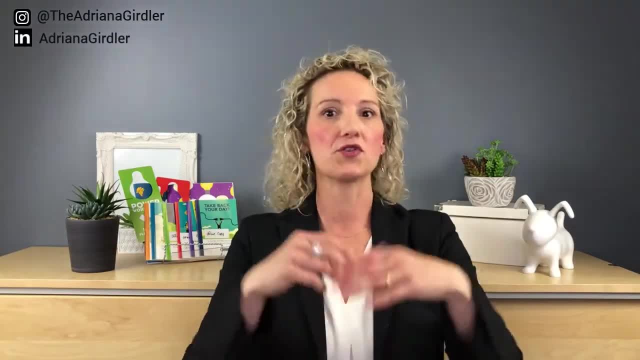 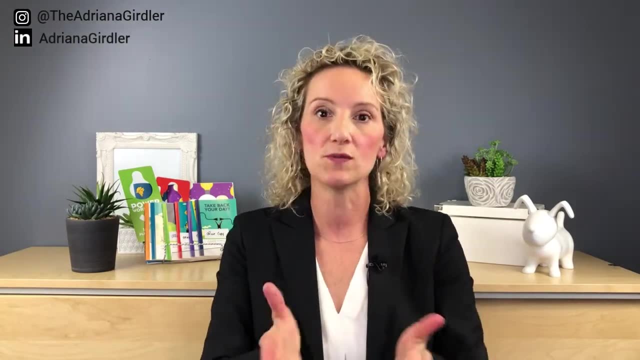 time where people are so focused on their to-do list for today that they're not taking a look at their calendar, And what I mean by this is you have to constantly take a look at your calendar from activities you have to do today, tomorrow, this week and even a month from now. And in my 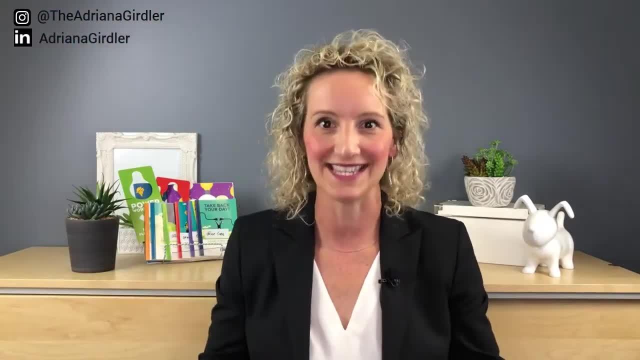 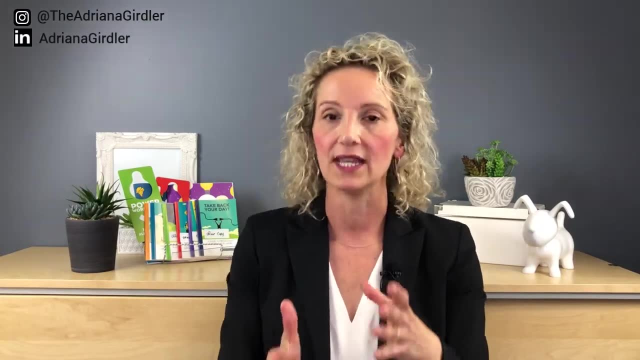 world. I actually look out months from now, sometimes going into the next year, So that, all being said, is when you're trying to be really productive and really manage your time effectively. you want to focus on your one to two goals that I said in the other tip, But you have to take into 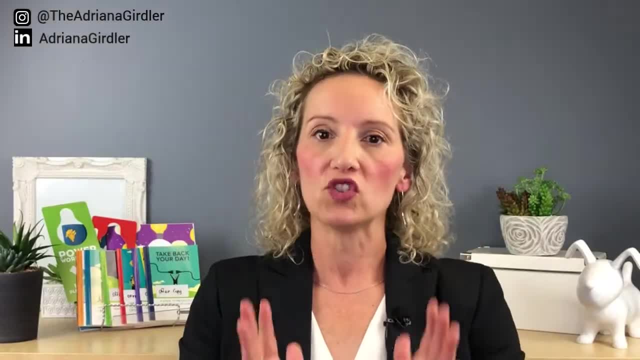 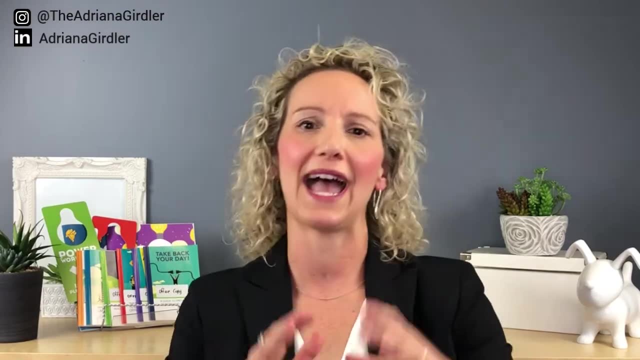 account what else is coming down the pike. So don't just focus on today. Integrate and look at your calendar so you can see what else you have to do, Because maybe just five minutes here or a half hour there in regards to those future activities can make a huge difference. because a little bit 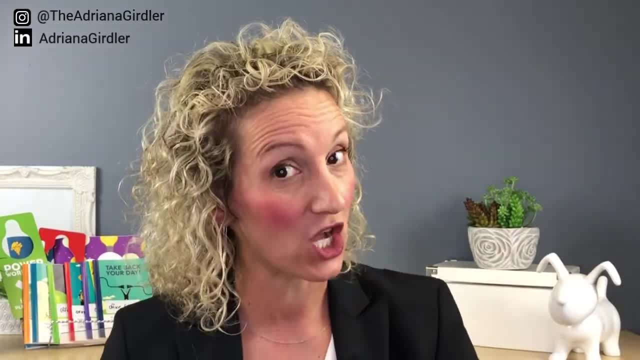 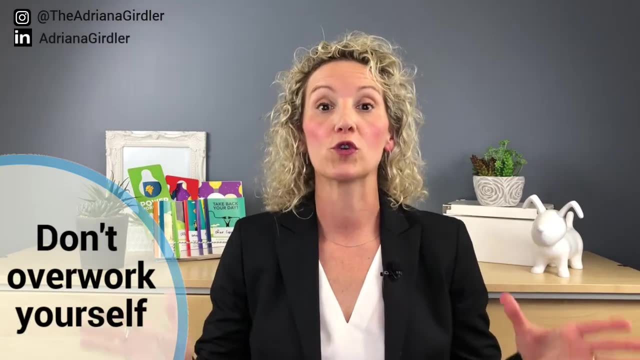 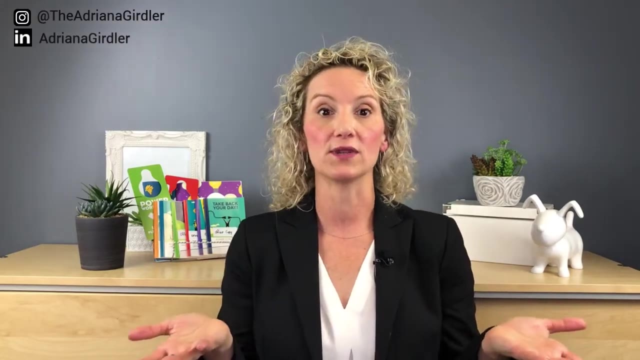 does go a long way. Are you ready to get back on track and not be overwhelmed? Write down less stress in the comments below. Don't overwork yourself. If you're going to be the master of your time and learn how to manage it properly, well then, you really got to take into account how you're working Stress levels. 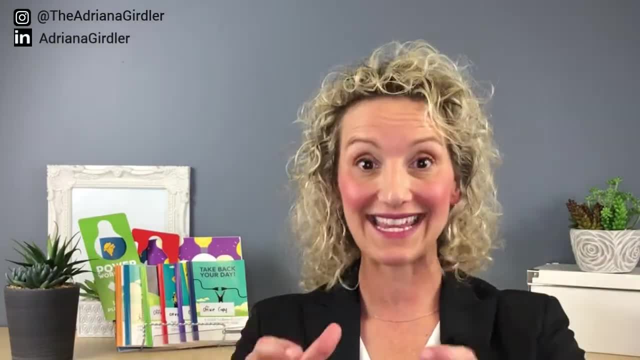 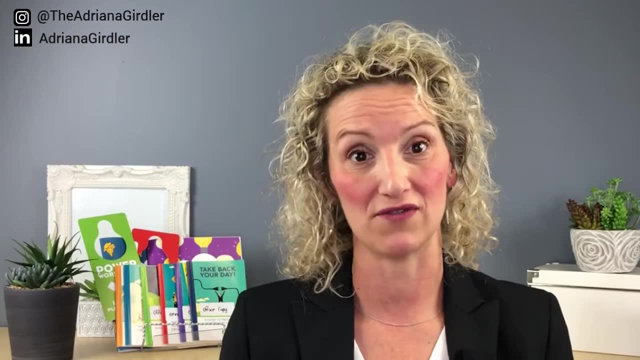 can get really high and you don't want to constantly be plugging in things that you have to do, So schedule in some rest time. That's really important. It's important to your wellbeing and your health and it's going to make a huge difference. Now, if you're saying to me: 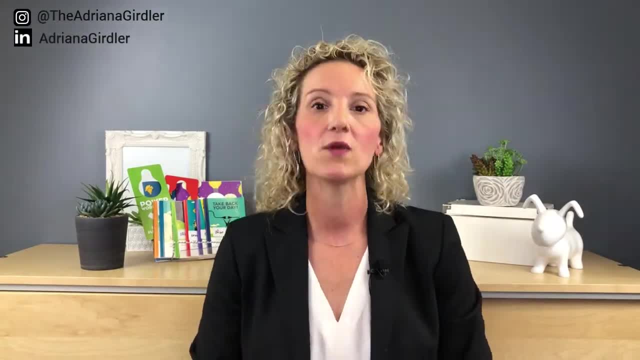 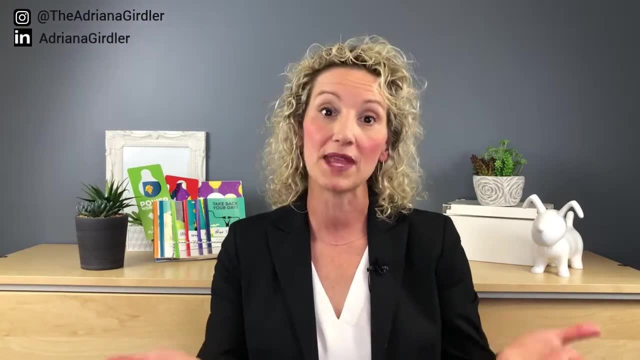 Adriana, I'm so busy I can't do it. I get it. You may want to put some rules into place, Like if you have kids, you're not going to check any of your emails till they go to bed. Okay fine, I get it. Or you may want to say: you know what The weekend. 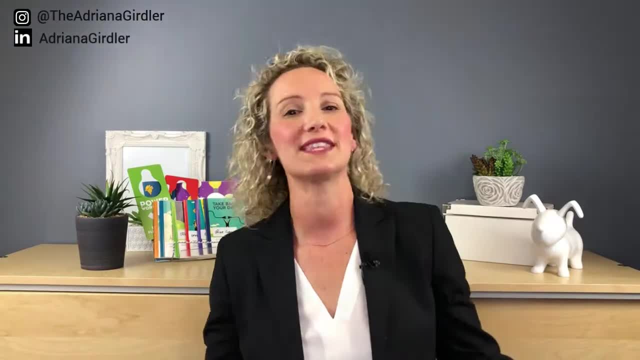 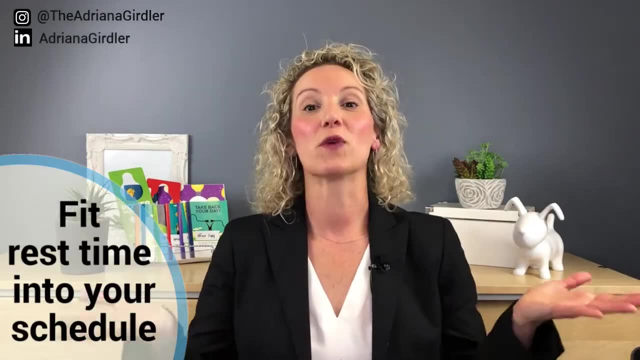 truly is my time. Saturday, there's nothing. Sunday: during the day, there's nothing. but on Sunday evening I'm going to prep for the following week. That's okay too, but you really got to balance it out. Fit rest time into your schedule. Have you ever heard of burnout? We all been there. 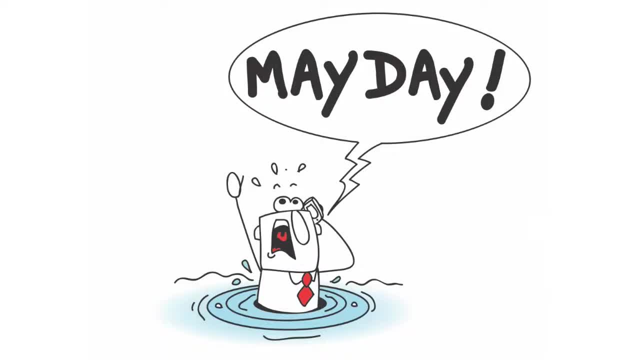 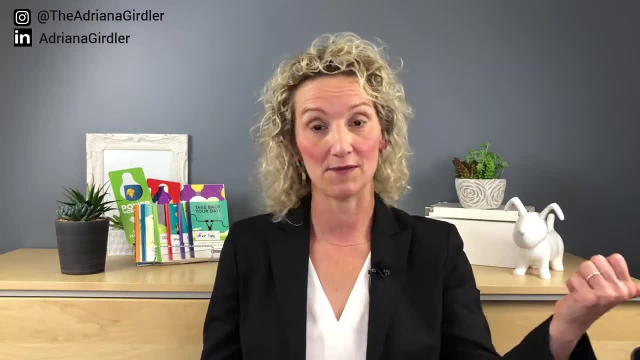 one time or another. If it hasn't been burnout at work, it's probably been burnout at home, because not only do we have these time commitments and obligations from a work perspective, if you have a family, I'm sure you have lots of them going on at home too. You got to schedule in some time for.